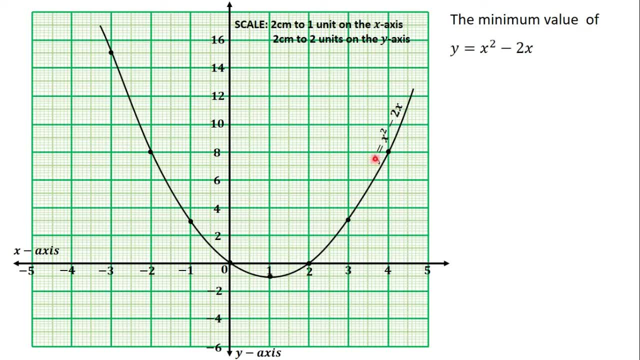 x. this is the graph of the relation. y is equal to s squared minus 2x. we are being asked to find the minimum value of y is equal to s squared minus 2x. as we learnt in the previous video, when the curve has a u-shape, the function will have a minimum value. so you see that here we are. 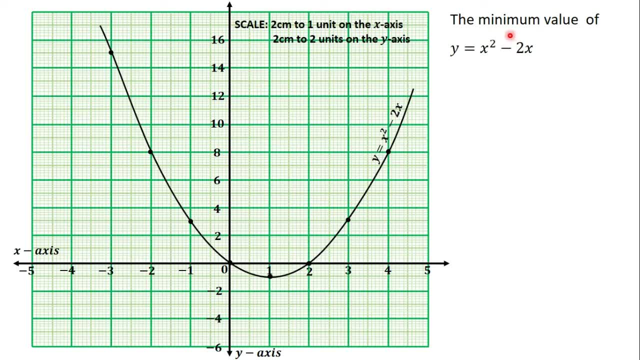 being asked to find the minimum value. the question could have said: we should find the least value, so the minimum value or the least value is the same thing. okay, we are going to use this graph to find the minimum value. of y is equal to s squared minus 2x. we learnt from the previous video that 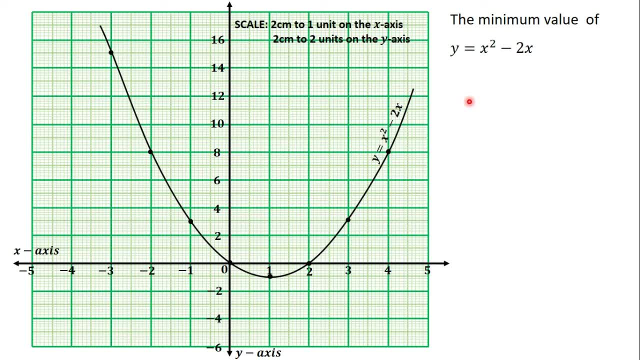 the minimum value is the y coordinates of the turning point. so to find the minimum value we first have to locate the turning point. as you can see, the turning point of the graph occurs here. to get the y coordinate you will trace it to the y axis. so we trace it to the y axis to get the y coordinates and from my graph, the 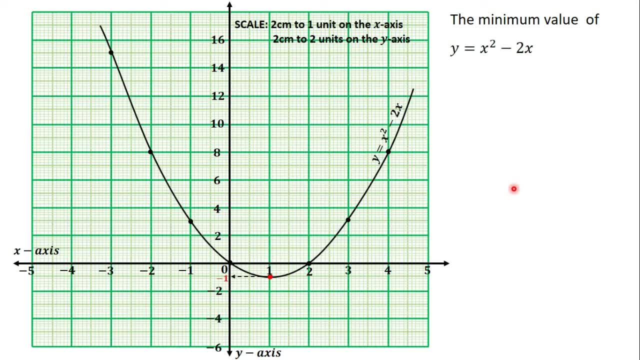 y coordinate here is minus 1.. so, from the graph, the minimum value of y is equal to s squared minus 2x is minus 1 and, as we can see, minus 1 is the smallest value of y that we have on this graph. let's move on to the next question. we have been asked to form a corresponding table of x and y. 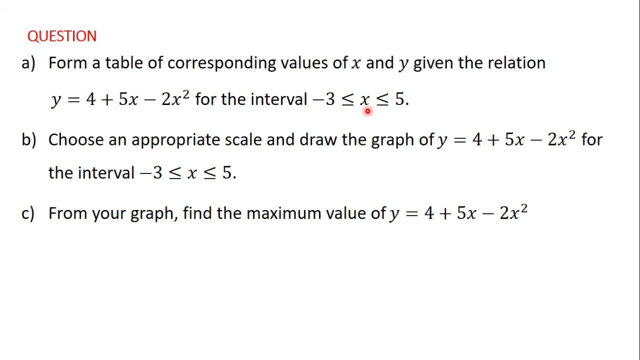 for this relation over this interval. then after that we use the points in the table to draw the graph of the relation. y is equal to 4 plus 5x minus 2 squared. then we'll use the graph to find the maximum value of 4 plus 5x minus 2 squared. so you move straight to the last part of our question. 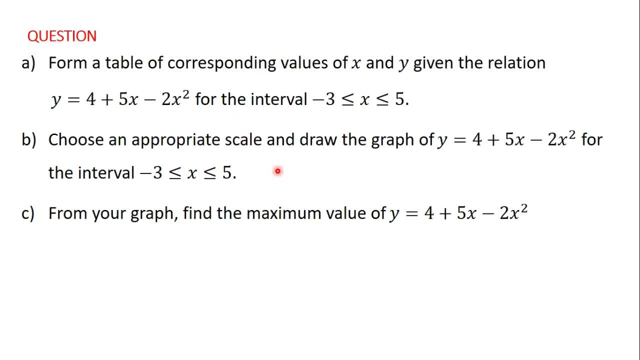 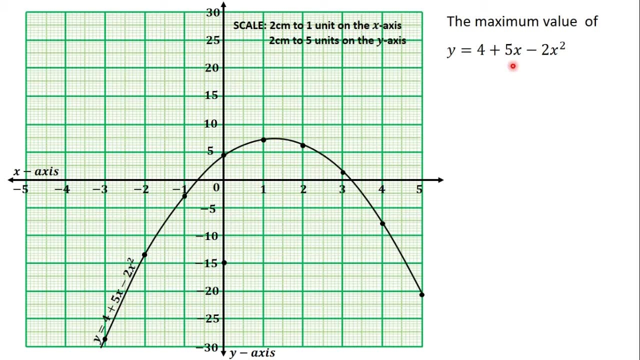 since we have already learned how to draw the graph of this relation, this is the graph of the relation. y is equal to 4 plus 5x minus 2 squared. we are going to find the maximum value, as we learned in the previous video. if the curve has an end shape like the one we have here, the function will have. 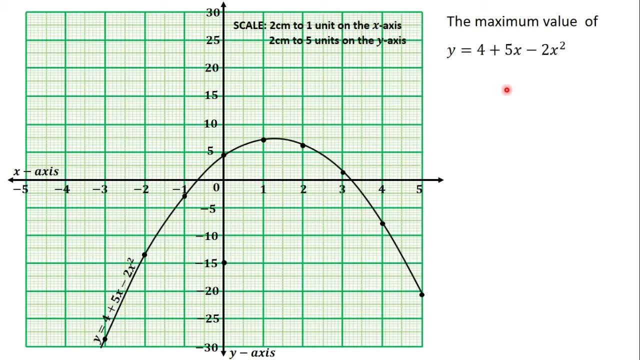 a maximum value. so to have maximum value or greatest value, the question could have said we should find the greatest value is the same thing, okay, so we are going to use the graph to find. the maximum value of y is equal to 4 plus 5x minus 2 squared. 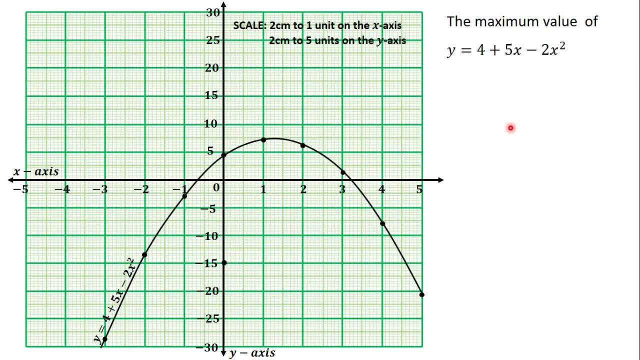 the maximum value is the y coordinate of the turning point. so the first thing we have to do is to locate the turning point. the turning point occurs here. then we will trace it to the y axis. so we trace it to the y axis and we read the y value there on my graph. the y value here is 7.5. 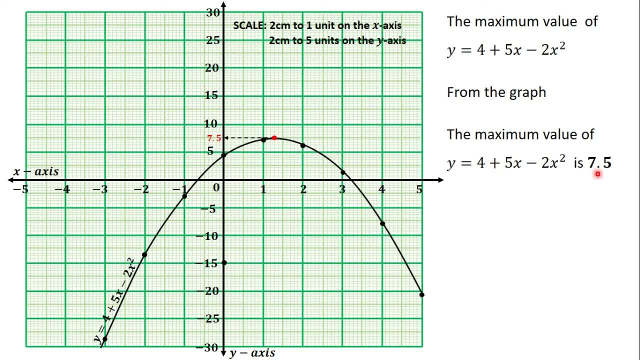 so from the graph the maximum value of y is 7.5 and we can clearly see that, because as soon as the curve gets to this point, it changes direction and starts moving downwards, so the y values decreases again. so from here the y values keeps on increasing, increasing, increasing. 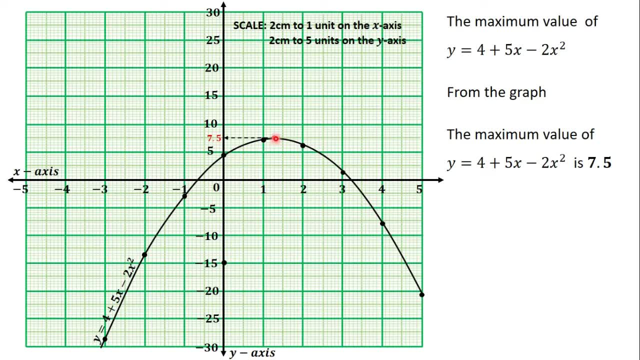 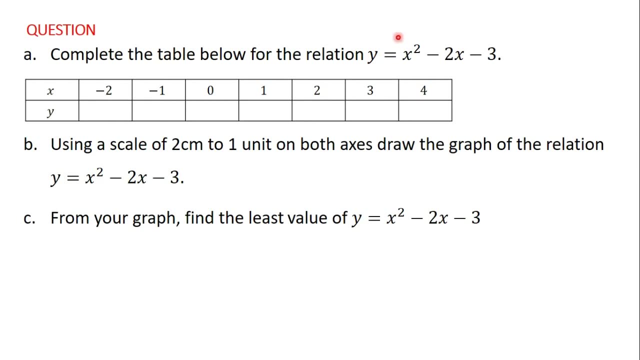 until it gets to the maximum value. then from the maximum value it starts decreasing again. so on this graph, the maximum value of y, or the greatest value of y, is 7.5. let's look at the next question. we have been asked to complete this table, for the relation, y is equal to s squared minus 2x minus 3. 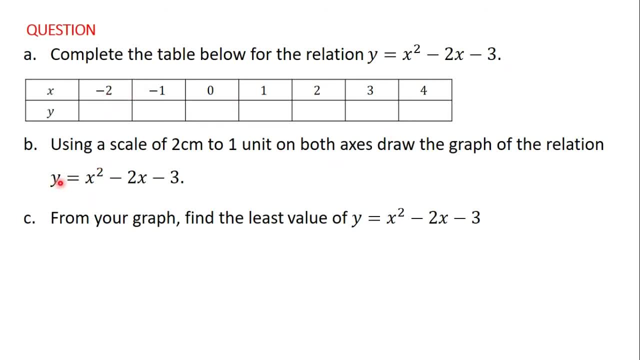 then we will use the points in the table to draw the graph of the relation. y is equal to s squared minus 2x minus 3. after that we will use the graph to find. the least value of y is equal to s squared minus 2x minus 3. the least value is also the same as the minimum value. so let's go to our graph sheet. 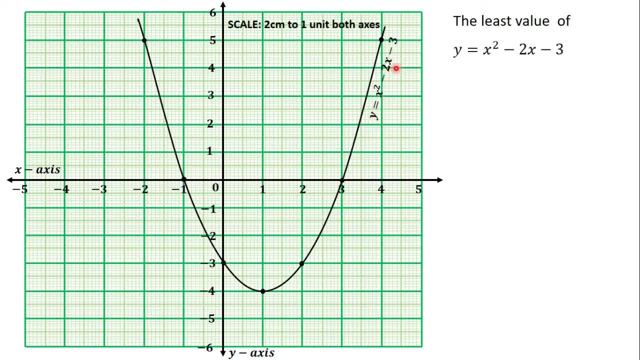 this is the graph of the relation. y is equal to s squared minus 2x minus 3. we are going to find the minimum value or the least value. as we learned in the previous video, if the graph has a u-shape, then the function will have a minimum value or a least value, so we are going to use this graph. 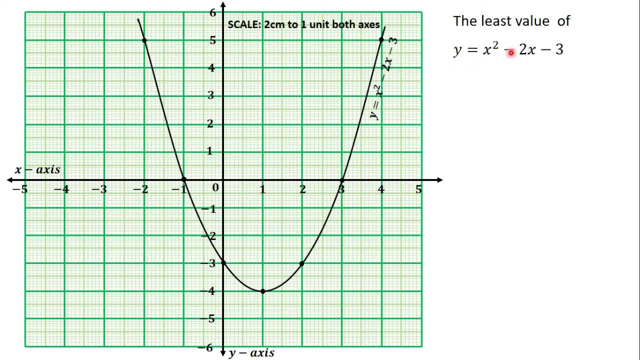 to find the least value or the minimum value of this function. to do that, we first have to locate the turning point, because the least value is the y coordinate of the turning point on the graph. this is the turning point. then, after we have located the turning point, we will trace it. 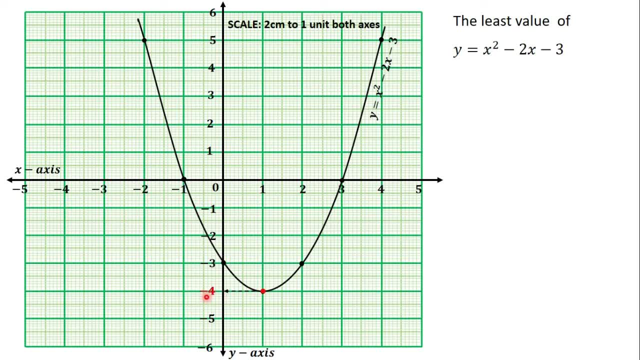 to the y axis. so we trace it to the y axis to get the y coordinate there, which is minus 4.. so from the graph the least value of y is equal to s squared minus 2x minus 3, s minus 4, and we 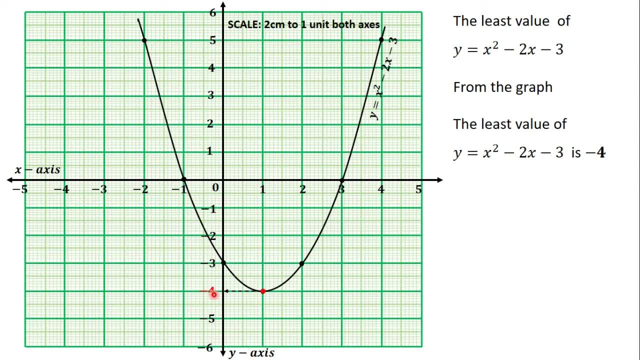 can clearly see that the least value or the smallest value of y on this graph is minus 4, because the curve starts from here and the y values keeps on decreasing as the curve moves downwards. so it keeps on decreasing until it gets to this point. then it changes direction. 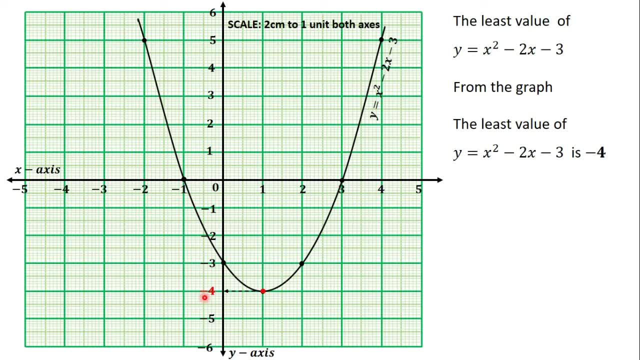 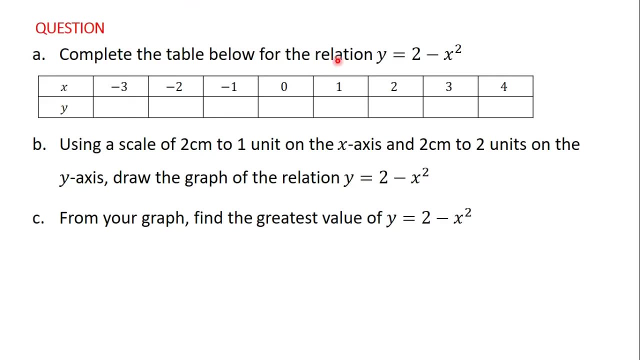 and it keeps on increasing again. so we can see that the smallest value of y, or the least value of y, is minus 4. so from this graph the least value of the function is minus 4.. let's look at the last question. complete the table below. for the relation, y is equal to 2 minus s squared. 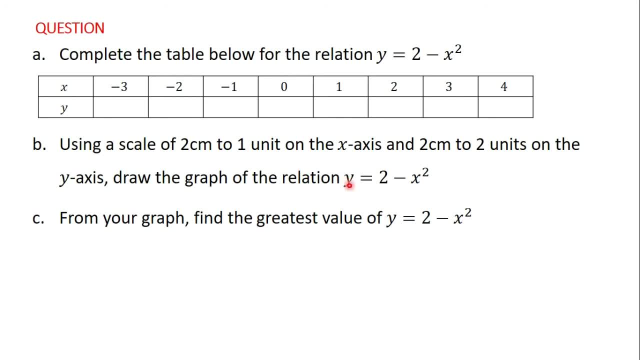 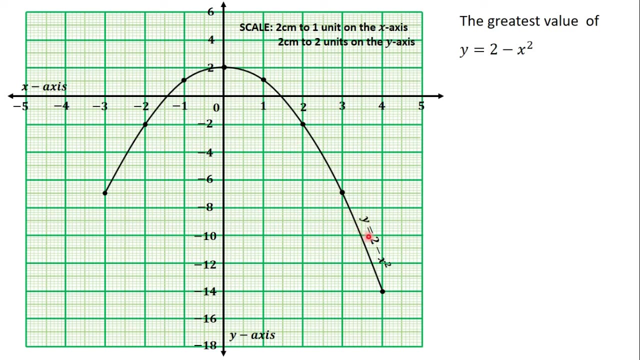 then we will use the points in the table to draw the graph of. y is equal to 2 minus s squared. after that we will use the graph to find the greatest value of y is equal to 2 minus s squared. so let's go to the graph sheet. this is the graph of the relation. y is equal to 2 minus s squared. 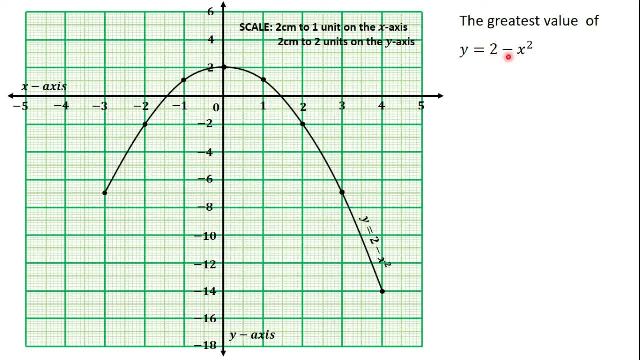 we are looking for. the greatest value of y is equal to 2 minus s squared. remember that the greatest value is the same as the maximum value and the curve will have a maximum value because it is having an end shape. the maximum value will occur at the turning point. so let's identify the turning point on the graph. it is this point here. 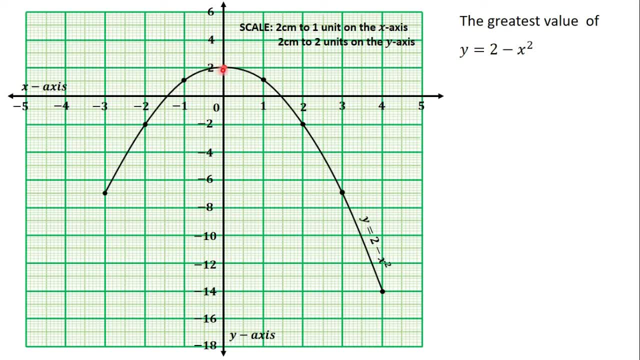 so this is the turning point. we will pick the y coordinate at the turning point. the y coordinate at the turning point is 2, so from the graph the greatest value of y is equal to 2 minus s squared is 2 and we can clearly see that the greatest value is 2 because the curve starts from.